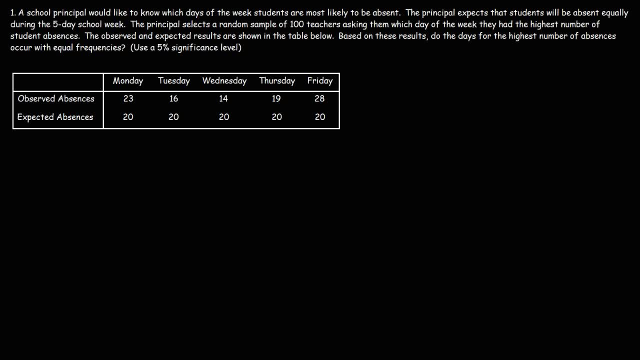 The principal expects that students will be absent equally during the five-day school week. The principal selects a random sample of 100 teachers, asking them which day of the week they had the highest number of student absences. The observed and expected results are shown in the table below. 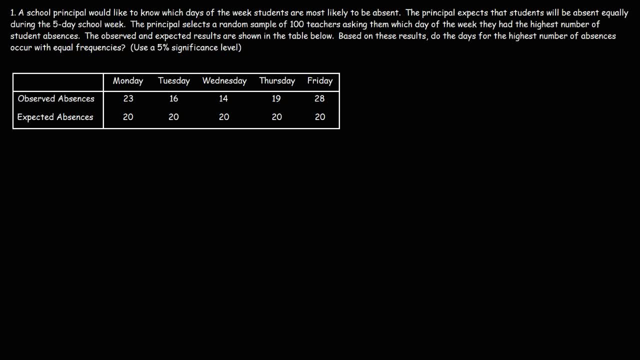 Based on these results, do the days for the highest number of absences occur with equal frequencies? What would you say? Use a 5% significance level to find out the answer. Now, the first thing we need to do is determine the null hypothesis and the alternative hypothesis. 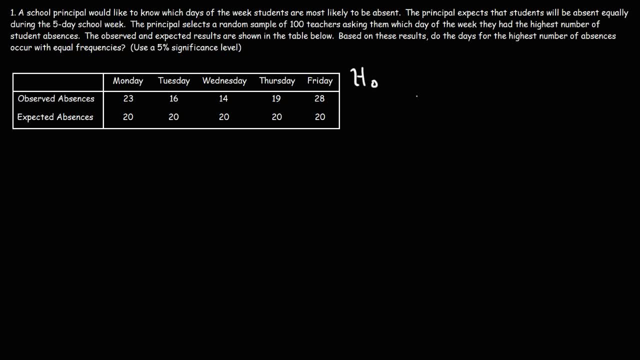 So for this problem the null hypothesis is that the absent days occur with equal frequencies, That is, they fit a uniform distribution. The alternative hypothesis is that the absent days do not occur with equal frequencies, Or rather they occur with equal frequencies. 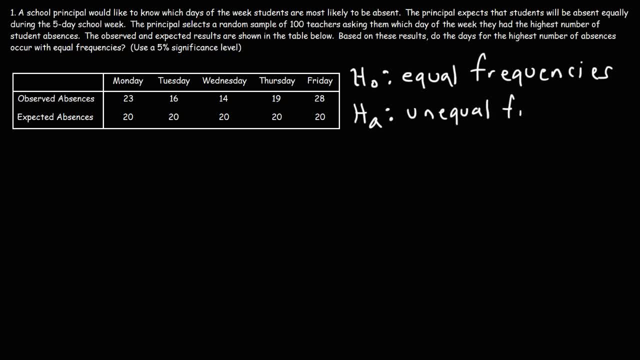 Or you could say that they don't fit a uniform distribution. Now, the goodness of fit tests is a right-tail test, And so I'm going to draw a graph. Now the chi-square. let me say that again: The chi-square distribution is not a symmetrical distribution. 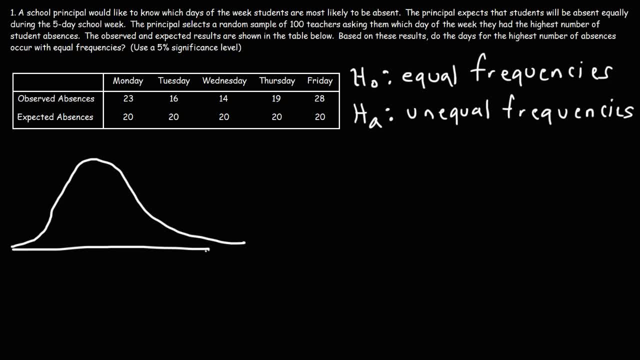 As you can see, it's skewed. This value here is known as the critical value, or rather the critical chi-square value. It separates the rejection region from the do-not-reject region. So this is the rejection region. I'm going to write rr to represent that. 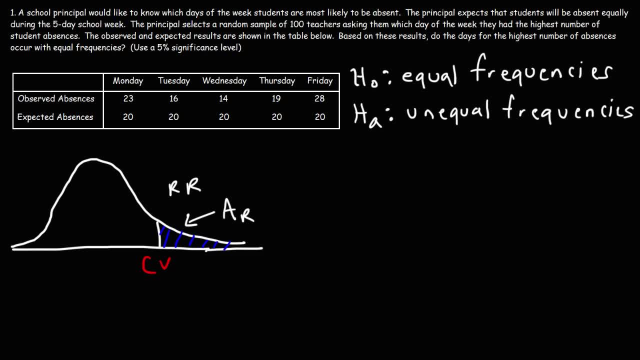 And the area shaded to the right of the critical value is going to be alpha, which in this case is 0.05.. The non-negative value is 0.05.. The non-negative value is 0.05.. The non-negative value is 0.05.. 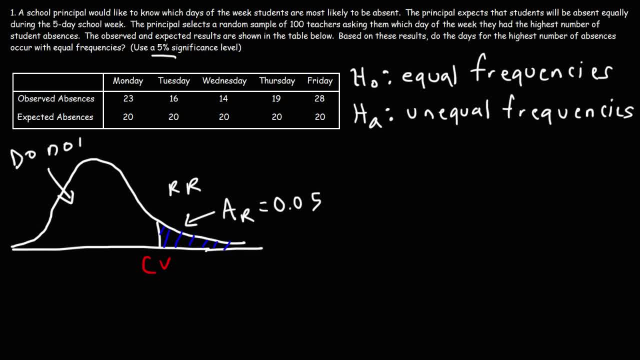 The non-shaded region is the do-not-reject region. So what we're going to do is we're going to get our calculated chi-square value, compare it to our critical chi-square value and see if the calculated value lies in the do-not-reject region or in the rejection region. 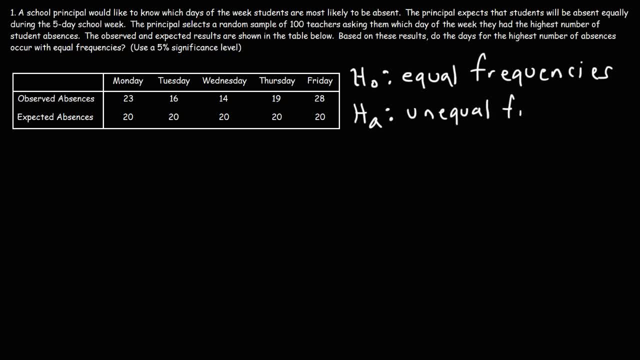 Or you could say that they don't fit a uniform distribution. Now, the goodness of fit tests is a right-tail test, And so I'm going to draw a graph. Now the chi-square. let me say that again: The chi-square distribution is not a symmetrical distribution. 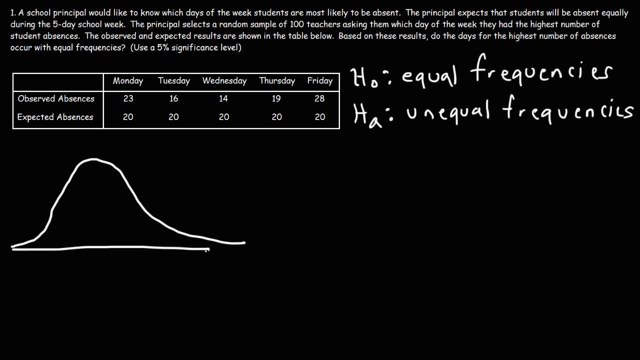 As you can see, it's skewed. This value here is known as the critical value, Or rather the critical chi-square value. It separates the rejection region from the do-not-reject region. So this is the rejection region. I'm going to write rr to represent that. 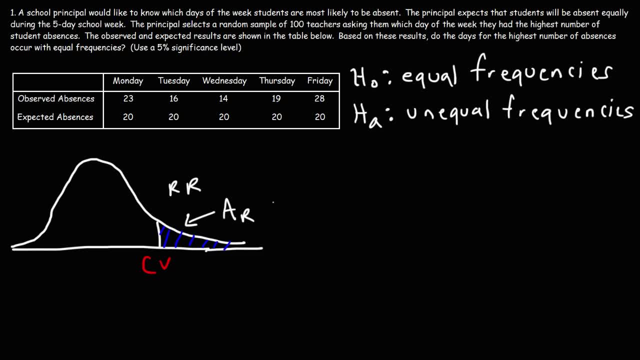 And the area shaded to the right of the critical value is going to be alpha, Which in this case is 0.05.. The non-negative value is 0.05.. And the non-negative value is 0.05.. So this is the non-negative value. 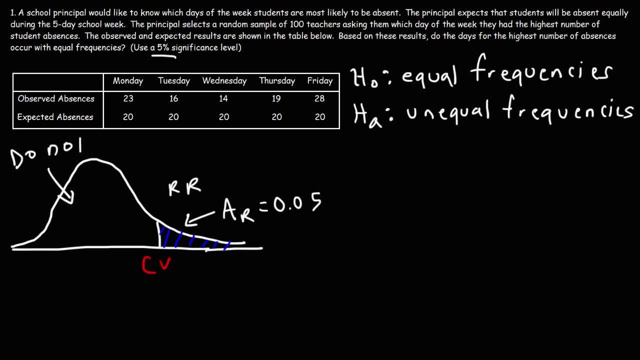 The non-shaded region is the do-not-reject region. So what we're going to do is we're going to get our calculated chi-square value, compare it to our critical chi-square value and see if the calculated value lies in the do-not-reject region. 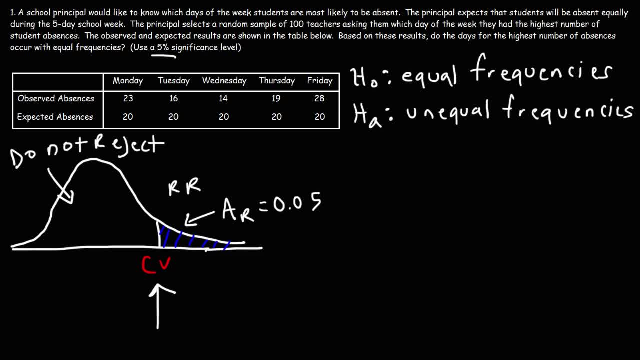 or in the rejection region. If it lies in the rejection region, we're going to reject the null hypothesis. Now let's begin by using the chi-square distribution table to get our critical chi-square value. So the first thing we need to do is determine the number of degrees of freedom. 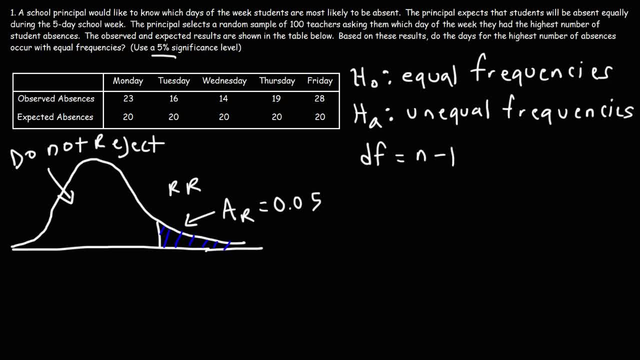 which is equal to n minus 1.. n is the number of categories our data is placed in, So the categories are the days of the week which we're using, 5 days of the week, So n is 5.. 5 minus 1 is 4.. 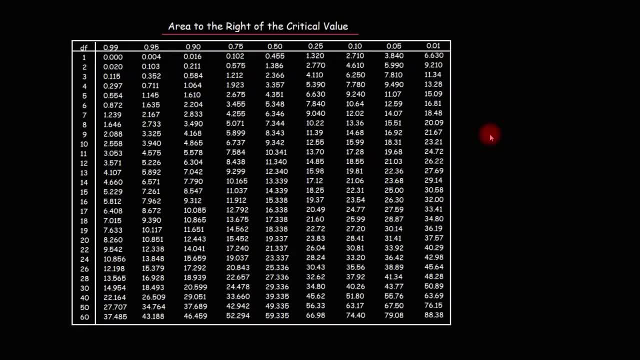 So we have 4 degrees of freedom. So here we have our chi-square distribution table And in the first column we have the degrees of freedom. In the first row we have the area to the right of the critical value And, as we said before, 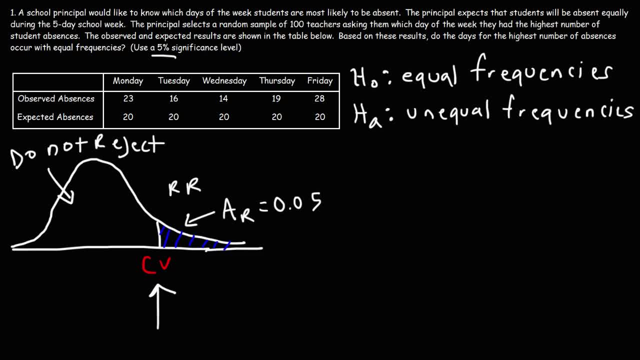 If it lies in the rejection region, we're going to reject the null hypothesis. Now let's begin by using the chi-square distribution table To get our critical chi-square value. So the first thing we need to do is determine the number of degrees of freedom. 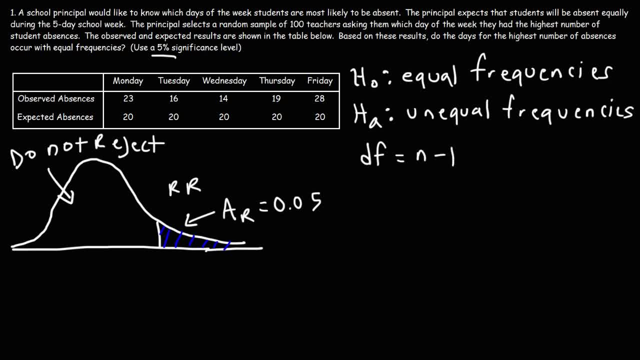 which is equal to n-1.. n is the number of categories our data is placed in, So the categories are the days of the week which we're using- 5 days of the week, So n is 5.. 5-1 is 4.. 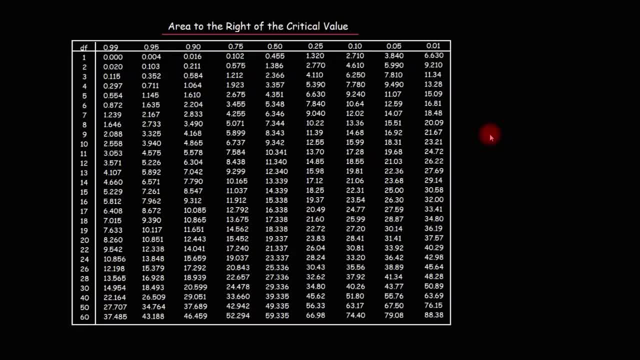 So we have 4 degrees of freedom. So here we have our chi-square value. So here we have our chi-square distribution table And in the first column we have the degrees of freedom. In the first row we have the area to the right, of the critical value. 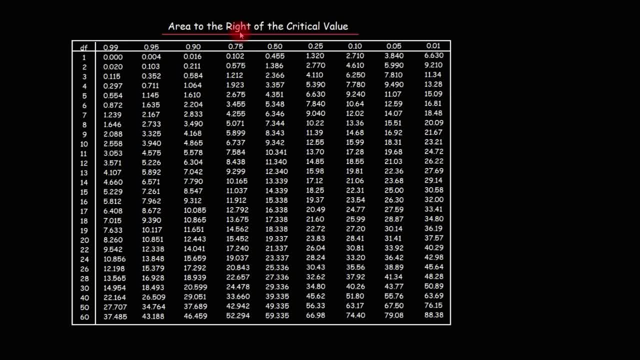 And, as we said before, the area to the right of the critical value for a right-tail test is alpha, which is 0.05.. So using this column- and we have 4 degrees of freedom- so using this row, we could see that our critical value is 9.49.. 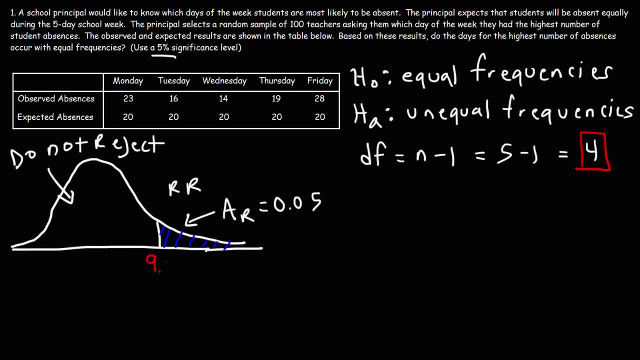 So let's place our critical value here And now we need to get our calculated chi-square value, And the formula that we're going to use is this formula: It's going to be sigma, which represents the sum of the difference between the observed values. 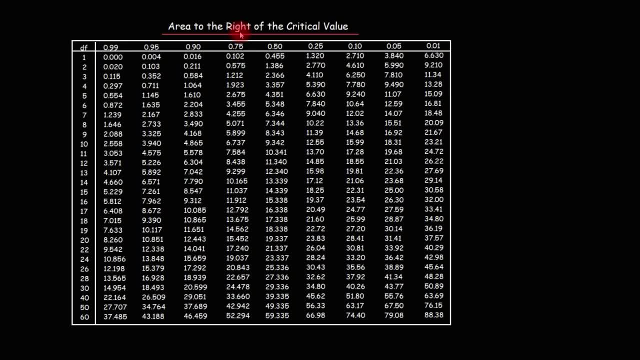 the area to the right of the critical value for a right-tail test is alpha, which is 0.05.. So using this column- and we have 4 degrees of freedom, so using this row, we could see that our critical value is 9.49.. 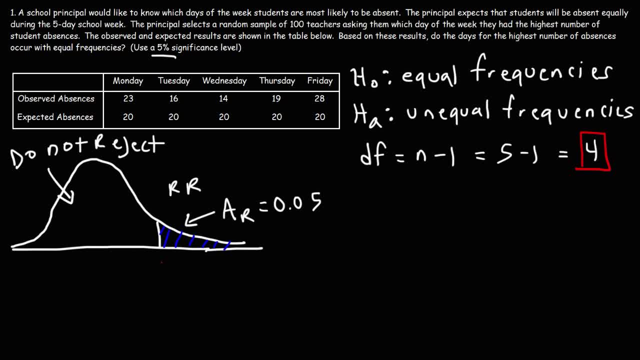 So let's place our critical value here And now we need to get our calculated chi-square value, And the formula that we're going to use is this formula: It's going to be sigma, which represents the sum of the difference between the observed values. 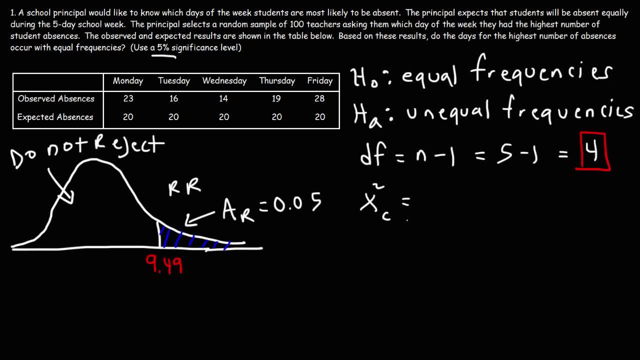 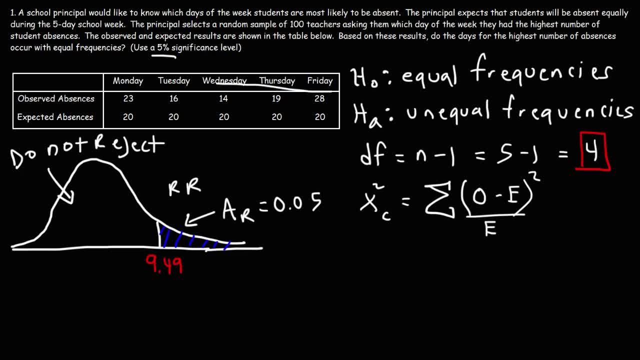 the first row is going to be: the first row is going to be: Sample contains the observed values, And the second one contains the expected values which have equal frequency. So, using this formula, here's what we're going to get. 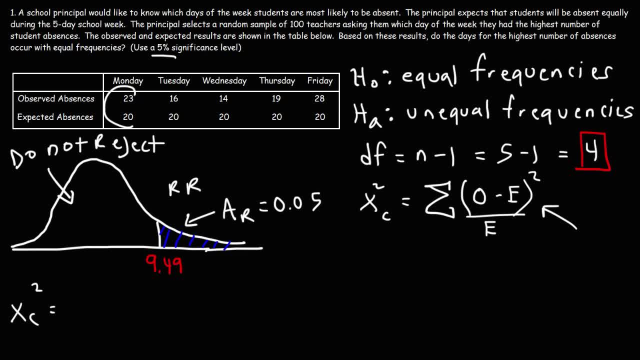 So, starting with Monday, if we take O subtracted by E, that's 23 minus 20, so that's going to give us 3 squared divided by the expected value of 20.. Next, for Tuesday, minus e, that's 16 minus 20, which is negative 4, but when you square it's. 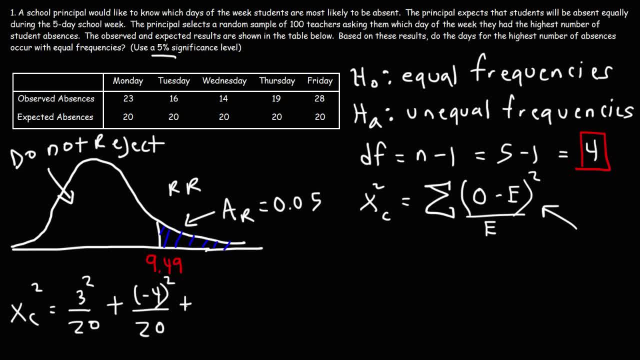 going to become positive. divided by e, which is 20, 14 minus 20, that's going to be negative 6. and next we have 19 minus 20, which is negative 1. and then for Friday we have 28 minus 20, which is positive 8. and then we just got to do: 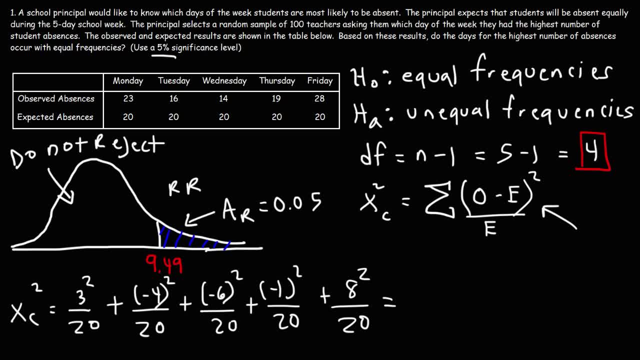 the math. so 3 squared plus 4 squared plus 6 squared plus 1 squared plus 8 squared, that's 126. so this is 126 divided by 20, which works out to be six point three. so this is our calculated chi-square value. so let's place that value on a. 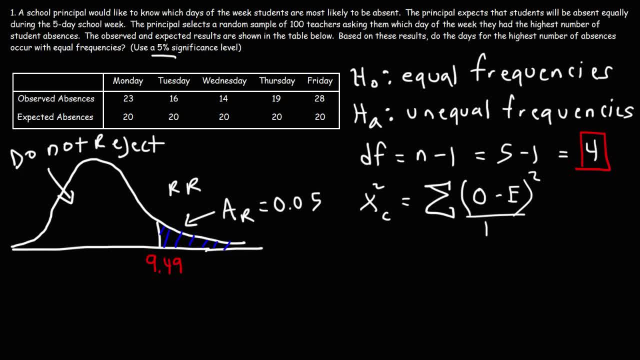 and the expected values squared, divided by the expected values, And we could find this in a table. The first row contains the observed values and the second one contains the expected values, which have equal frequency. So, using this formula, here's what we're going to get. 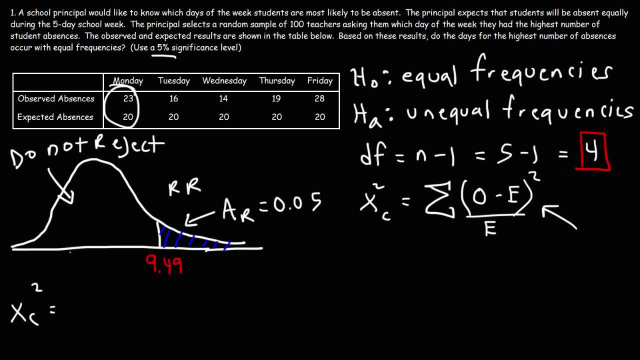 So, starting with Monday, if we take O subtracted by E, that's 23 minus 20, so that's going to give us 3 squared divided by the expected value of 20.. Next for Tuesday: O minus E, that's 16 minus 20,.